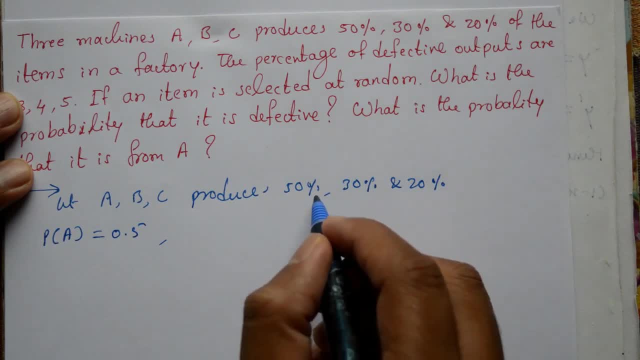 That is 0.5. aayega Baadme probability of B machine B kitna produce karo hai 30%, karo hai 30 by 100, that is 0.3 hota hai And the probability of C 20% hai. That is: 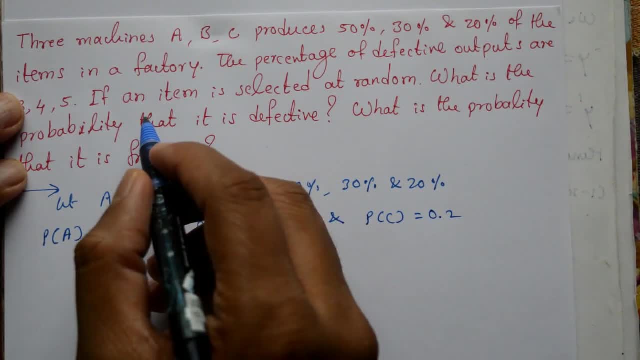 0.2 hota hai Now. so kya hai? The percentage of defective outputs are 3,, 4,, 5,, 6,, 7,, 8,, 9,, 10,, 11,, 12,, 13,, 14,, 15,, 16,, 17,, 18,, 19,, 20,, 21,, 22,, 23,, 23,, 24,. 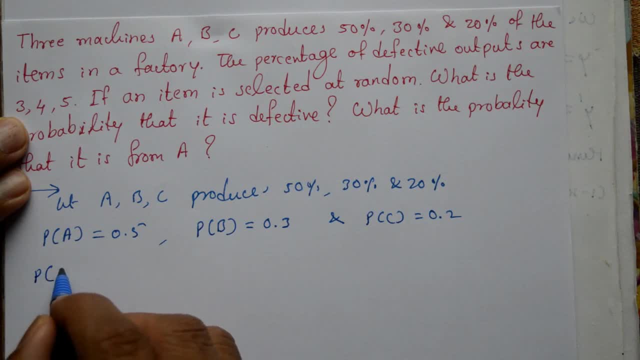 25 hai. That is the probability of defective A. that is 3 hai 3 percent hota hai. That is 0.03 aayega. And the probability of D by B hai Second machine: 4 percentage, 4 percentage. 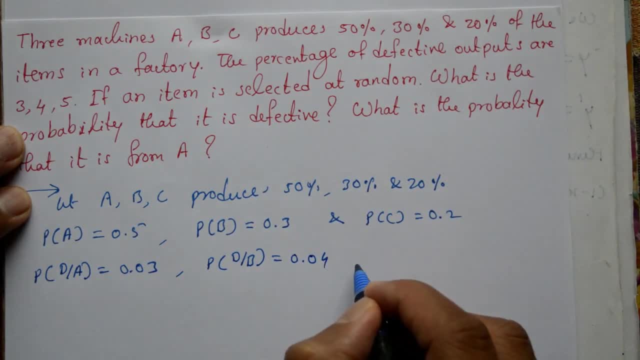 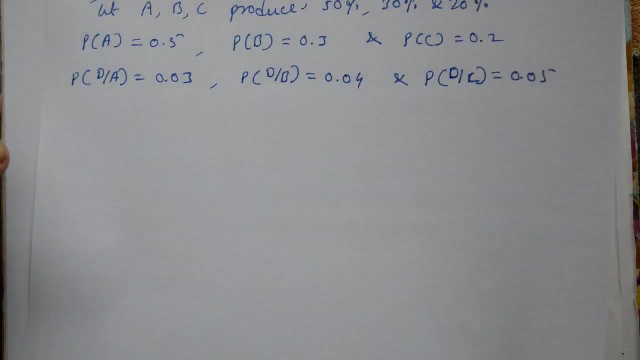 hai, That is 4 divided by 100, 0.04 ho jayega. And the probability of C slash B- sorry, D slash B is C is equal to. is that correct? 5 percentage: 5 divided by 100, ho jayega, that is 0.05 aayega. Now, so D, kya hai there? D denote D means: 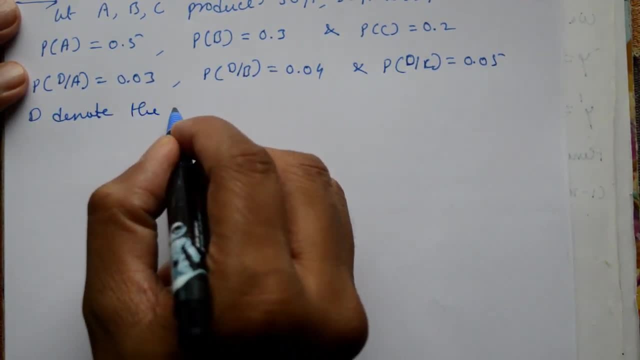 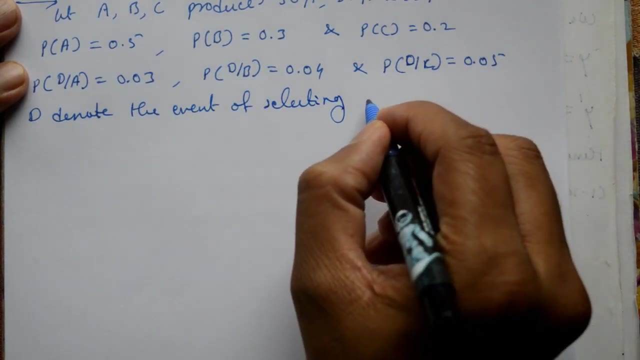 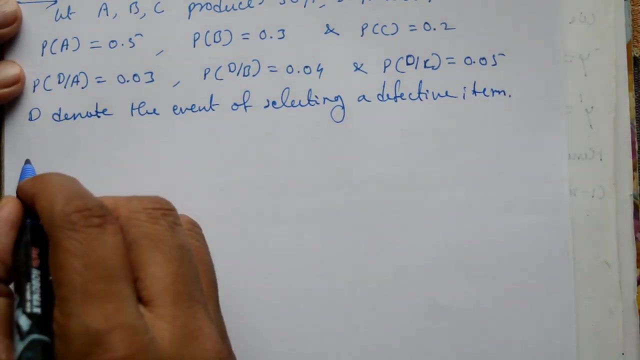 say: kya hai na. So what is D? D denote the event of selecting a defective item, of selecting a defective item. A. ok. So what we want to do? What is the probability that it is defective? karke hai. That is the. 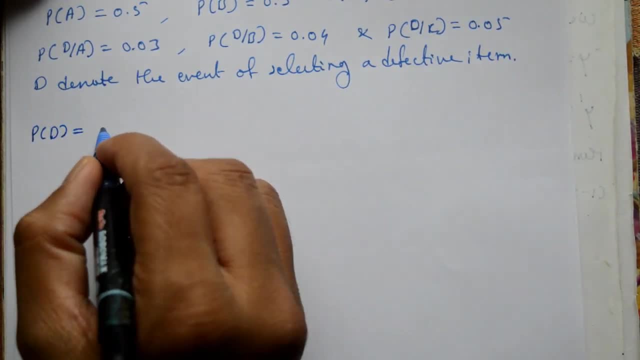 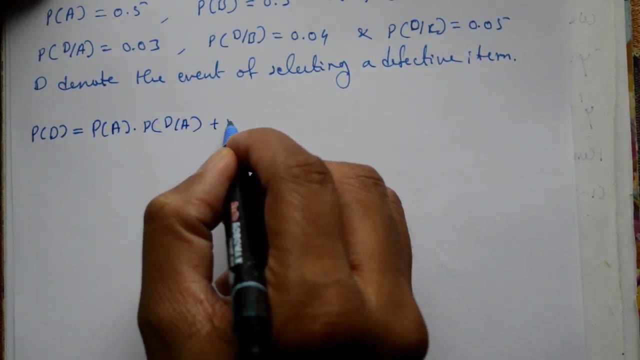 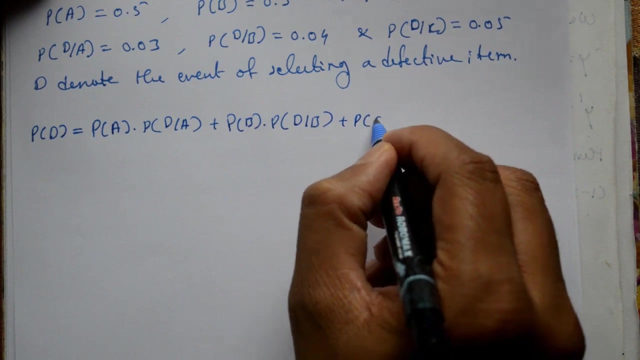 probability of D is equal to. the probability of D is equal to aayega. the probability of probability of A into probability of D slash A, plus probability of B into probability of D slash B- aayega, plus probability of C into probability of D slash C- aayega. And. 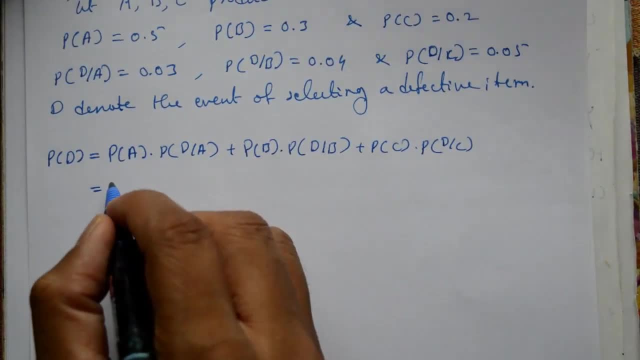 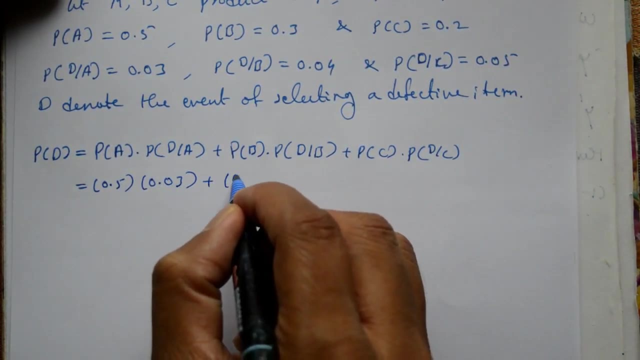 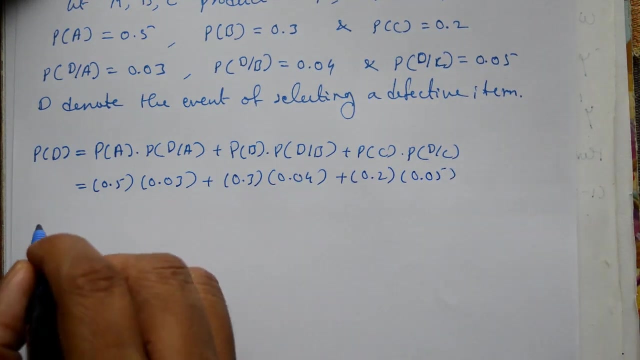 that is equal to either value. say subsequent value. Thank you very much. 0.5 into that is a 0.03 plus 0.3 into 0.04 plus 0.2 into 0.05.. The probability of D that is equal.